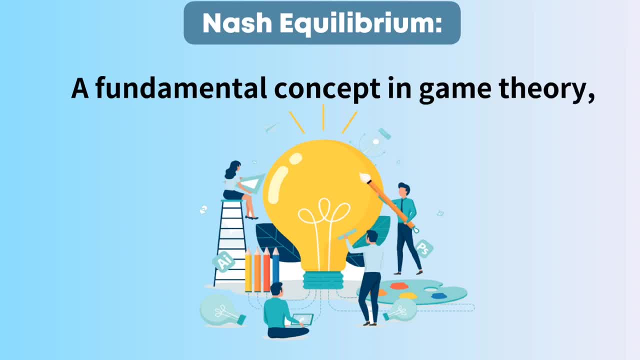 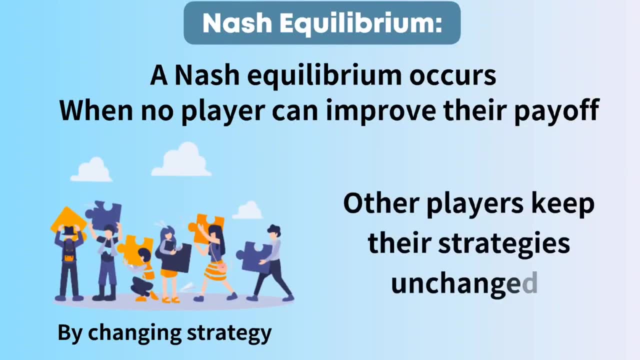 Nash equilibrium, a fundamental concept in game theory. A Nash equilibrium occurs when no player can improve their payoff by changing their strategy, while the other players keep their strategies unchanged. In other words, it represents a stable state where no one has a chance to win. In other words, it represents a stable state where no one has a chance to win. In other words, it represents a stable state where no one has a chance to win. The Roman formula stores an incentive to deviate celebratory or not celebratory for any engagement. Rather, it is often criticized as an incentive to deleviate. 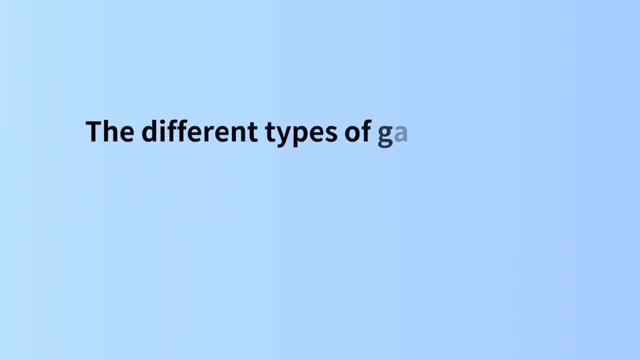 The Roman formula stores an incentive to develop. divided into three categories. Theías scalability is used to simplify normal rule of reactivity, majorinde. The different types of game theory are as follows: modular capitalism is interesting. 1. 1. cooperative & noncooperative. 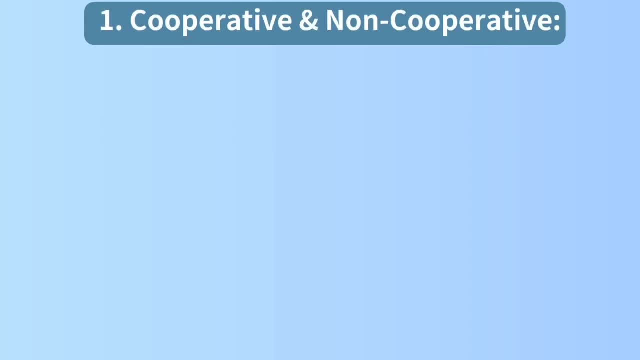 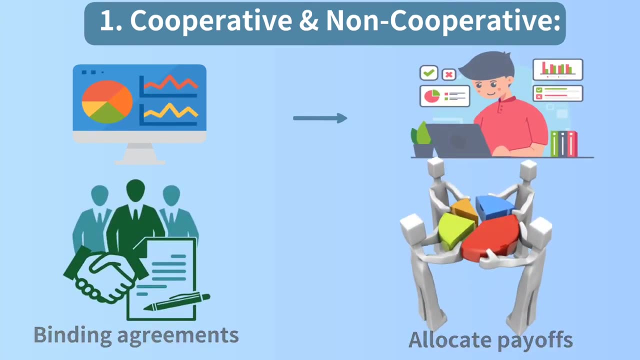 type of game theory, only the one who exists. This analysis involves studying how players form binding agreements. Each stunts independent from other players and allocates payoffs between themselves. player who give psychopathic zulse: each counter is led by the inherent. the non-cooperative game is captivating. 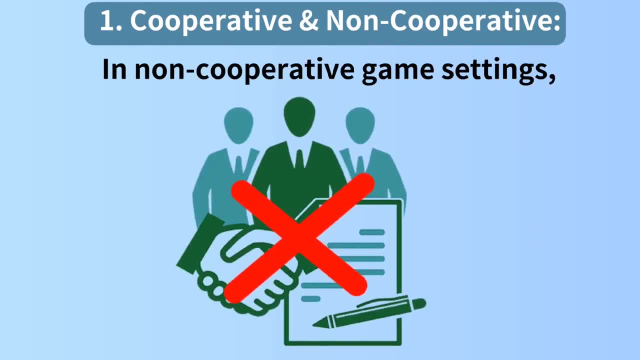 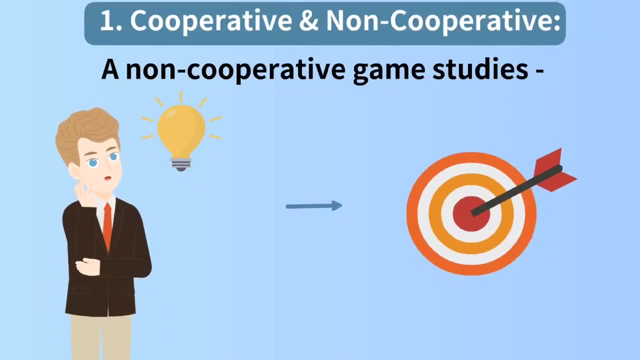 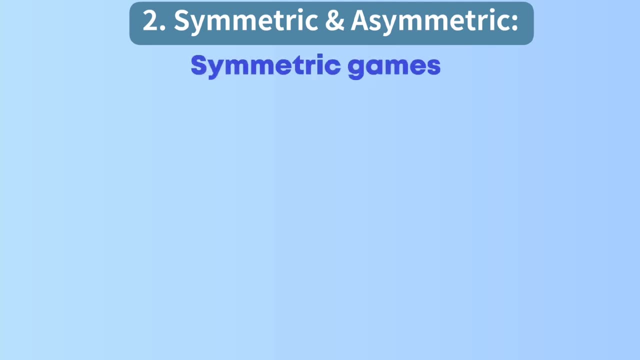 In non-cooperative game settings, Players cannot get into binding agreements. A non-cooperative game studies how rational individual players game studies how rational individual players decide their strategy to fulfill their objectives. 2. Symmetric and Asymmetric. In the case of symmetric games, the payoffs depend on each player's strategy. 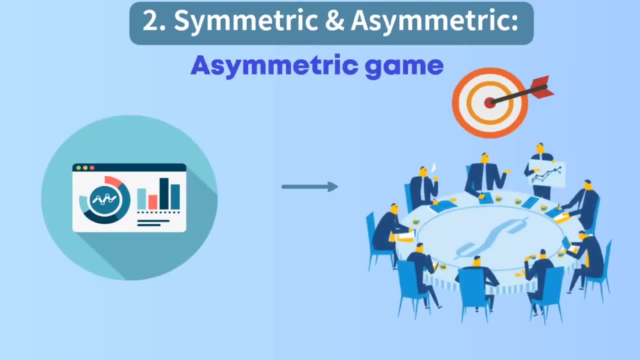 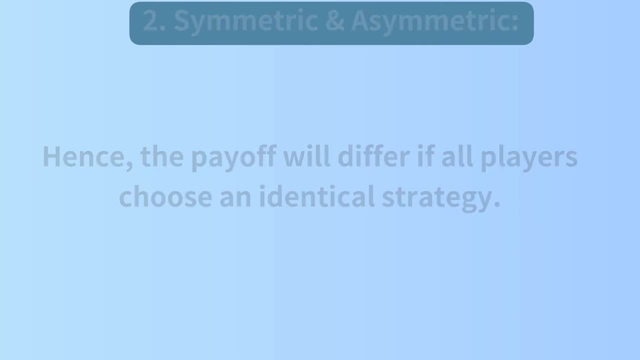 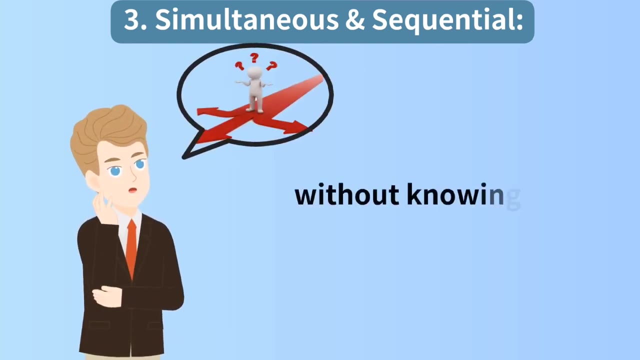 Conversely, in asymmetric game settings, the payoffs vary among the players. Hence the payoff will differ if all players choose an identical strategy. 3. Simultaneous and Sequential. A game where players make a decision without knowing other players' decisions or all players make their decision simultaneously is a simultaneous game. 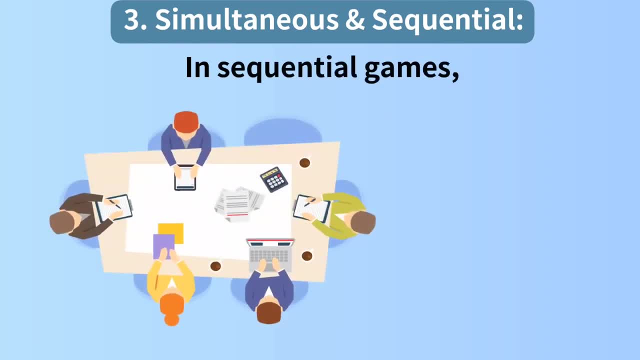 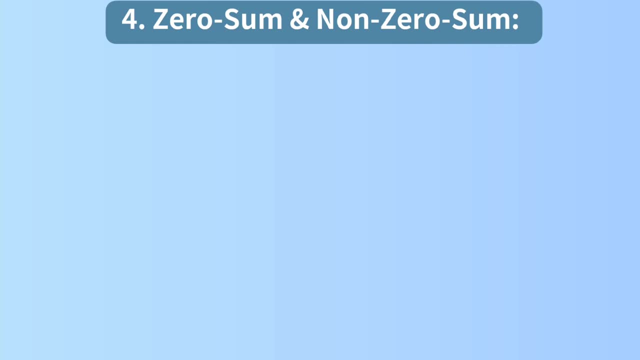 In sequential games, players are aware of the other players' decisions or they take turns to decide. 4. Zero-Sum and Non-Zero-Sum. In zero-sum games, a participant's gains or losses balance other participants' gains or losses. 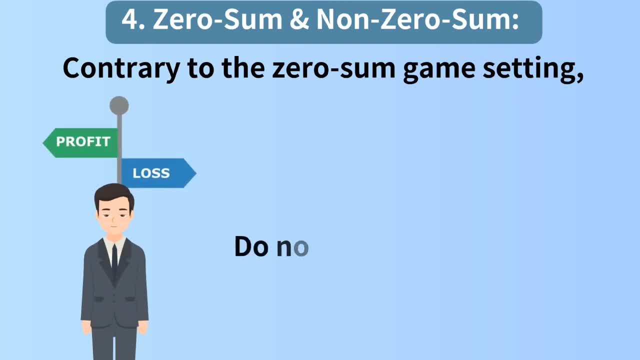 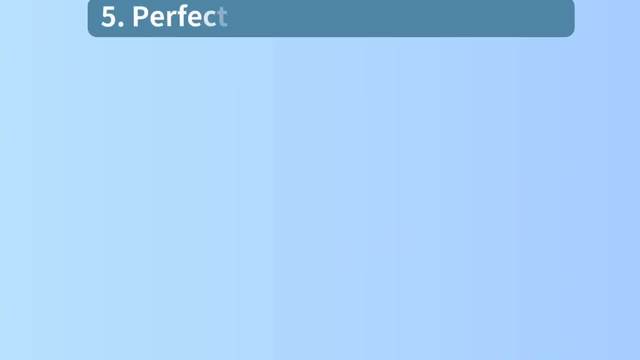 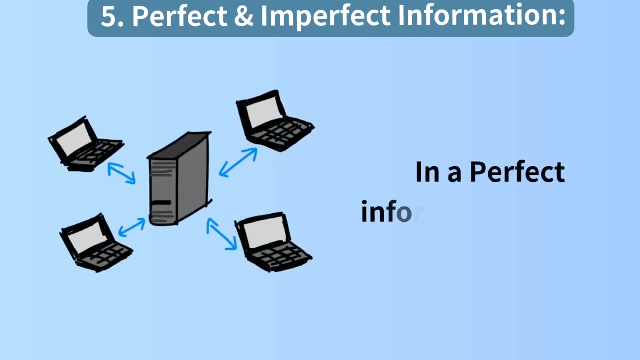 Contrary to the zero-sum game settings, a player's gains or losses do not result in other players' gains or losses in a non-zero-sum game. 5. Perfect Information and Imperfect Information. All participants have access to the same information in a perfect information setting. 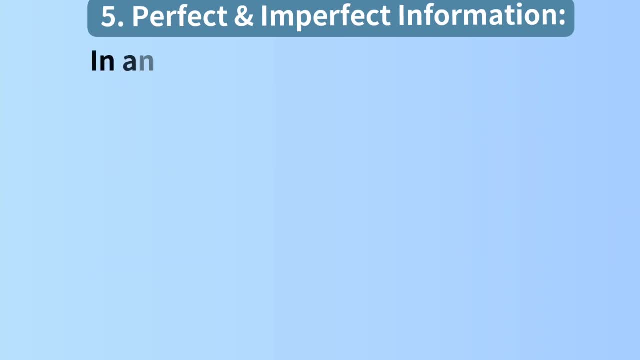 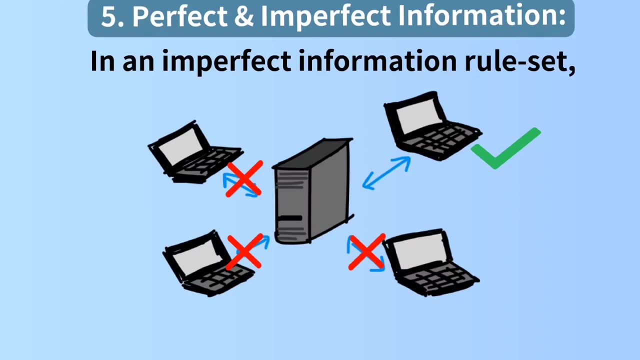 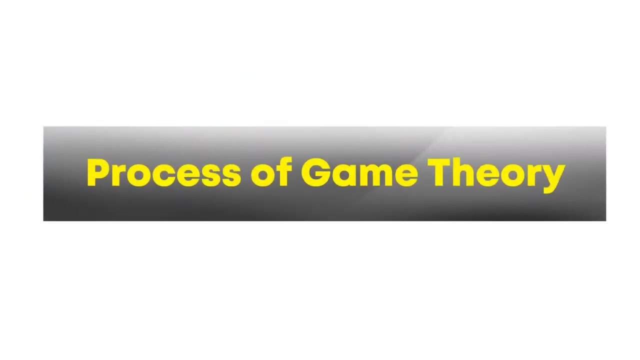 Therefore, they make their decision based on the data. However, in an imperfect information rule set, the data available to one player is unavailable to other participants. Please like the video? Thanks. Process of game theory. Here's a general process of applying game theory in operations management. 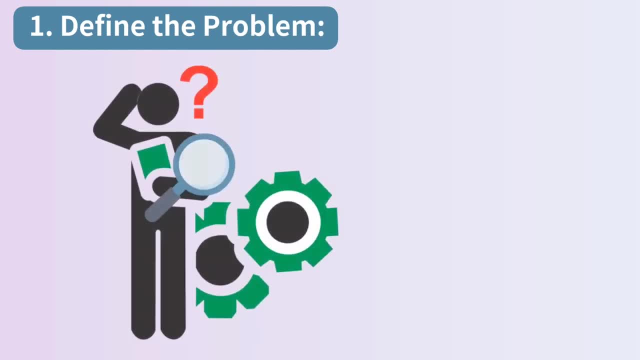 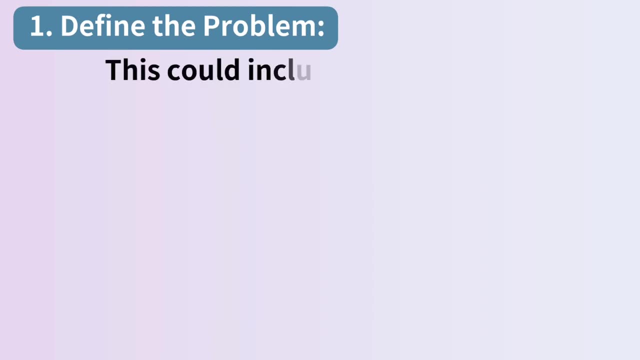 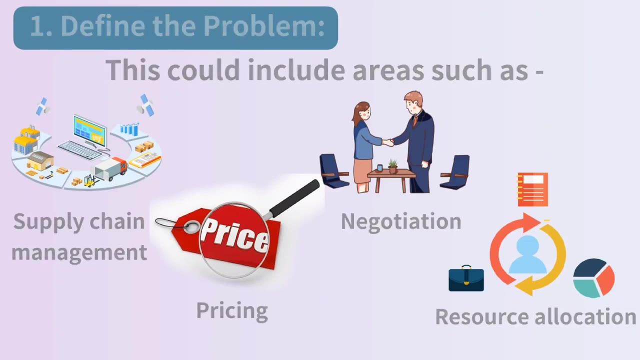 1. Define the problem. Begin by identifying the specific problem or decision making scenario within your operations that you want to address. This could include areas such as supply chain management, pricing negotiation, resource allocation and more. 2. Identify parameters- the players- Determine who the relevant players or stakeholders are in the given scenario. 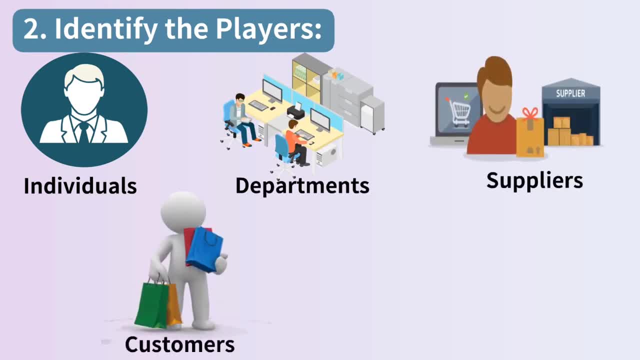 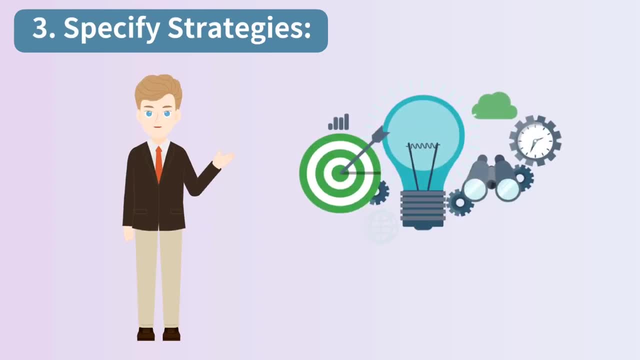 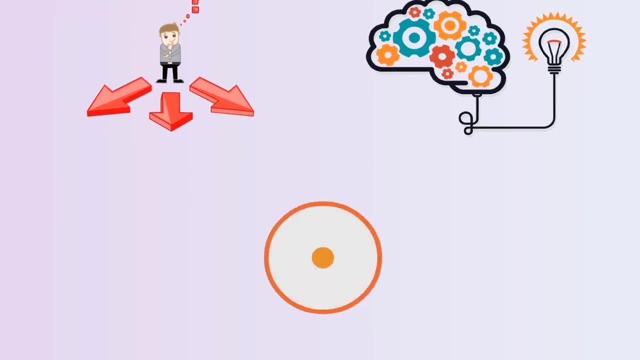 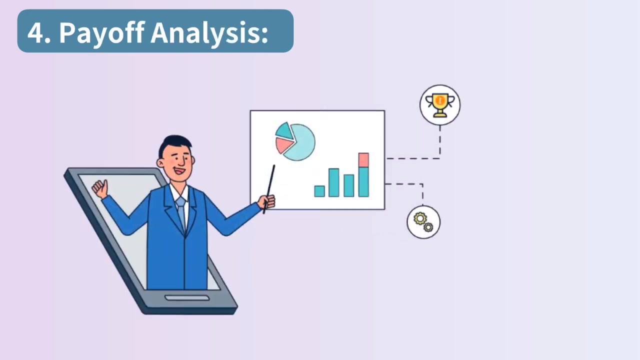 This could be individuals, departments, suppliers, customers or competitors. 3. Specify strategies: Define the possible strategies that each player can adopt. These strategies represent the available choices or actions they can take to achieve their goals within the context of the problem. 4. Payoff analysis: Assign numerical. 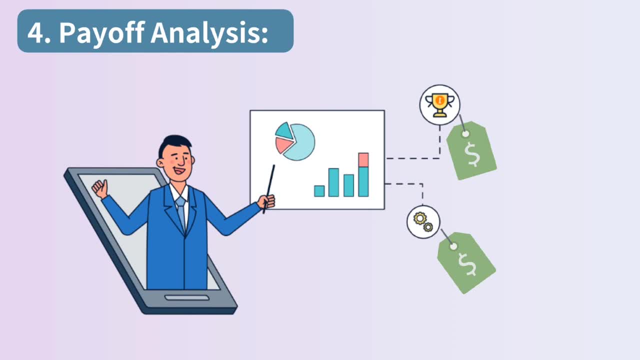 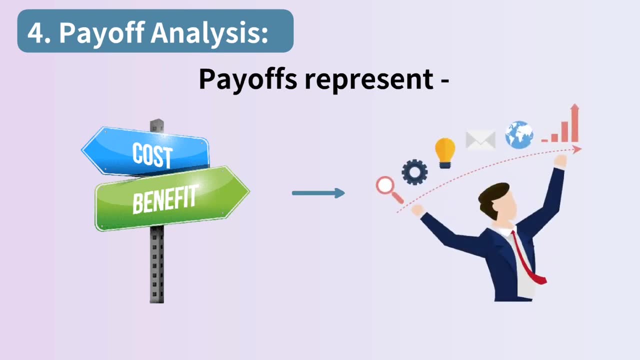 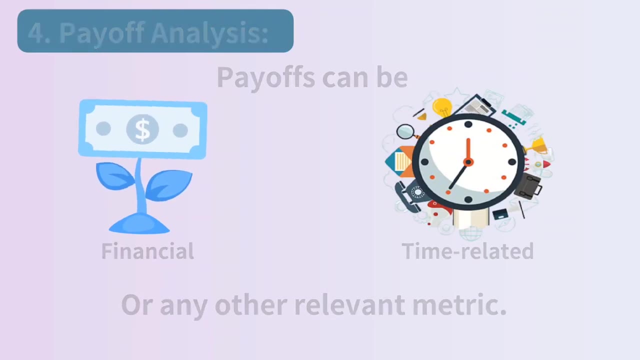 payoffs or utility values to each possible outcome of the game. Payoffs represent the benefits or costs associated with the various combinations of strategies chosen by the players. Payoffs can be financial, time-related or any other relevant metric. 5. Model the game. Choose an appropriate game theory model to 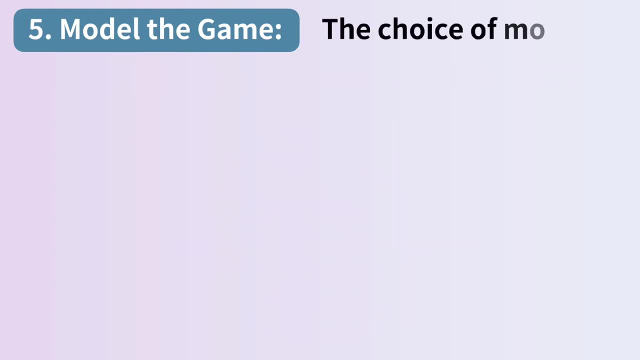 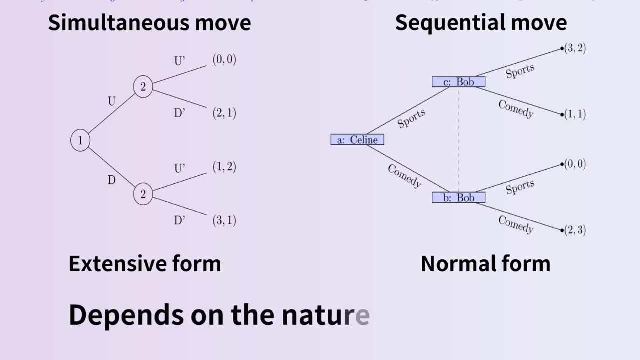 represent the game. 4. Payoffs Assign numerical payoffs or utility values to each possible outcome of the game. Payoffs represent the strategic interactions. The choice of model- for example, simultaneous move, sequential move, extensive form, normal form- depends on the nature of the problem. 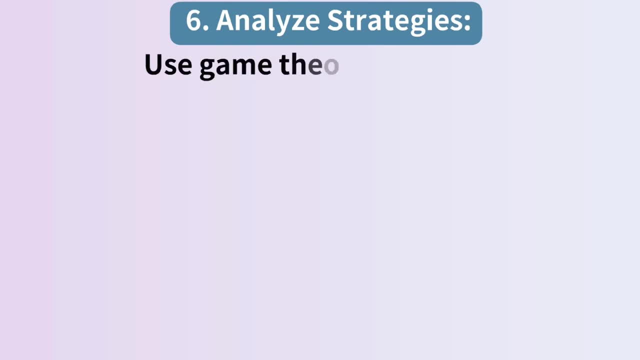 6. Analyze strategies: Use game theory concepts to analyze the strategies and outcomes. Identify potential Nash equilibria, which are situations where no player can improve their payoff by changing their strategy. 7. Sensitivity analysis: Assess how the outcomes change as you vary the payoffs. 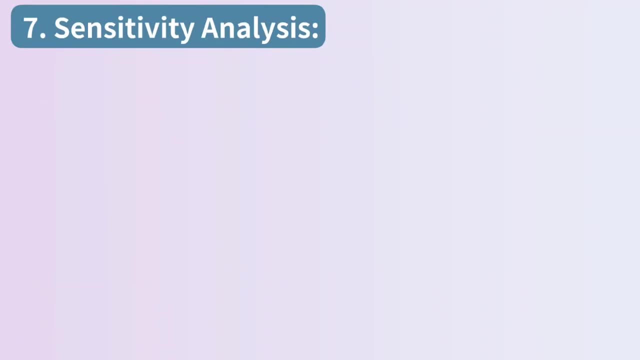 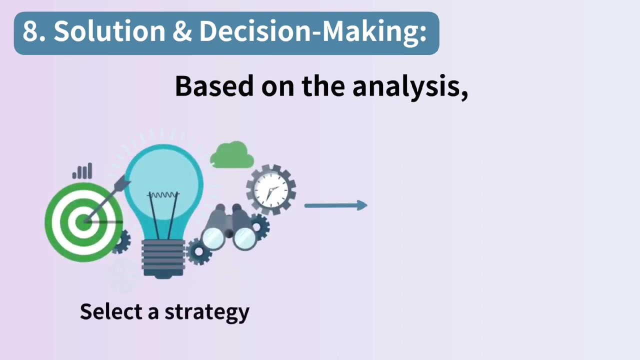 strategies or assumptions in the game. Sensitivity analysis helps in understanding the robustness of the strategies and the potential risks. 8. Solution and decision-making: Based on the analysis, select a strategy or a combination of strategies that best aligns with the organization's objectives. The chosen strategy may involve cooperation. 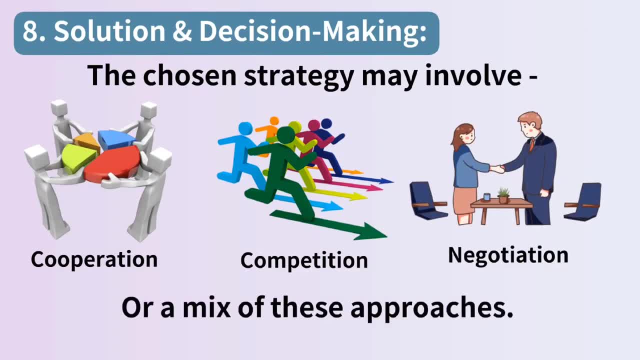 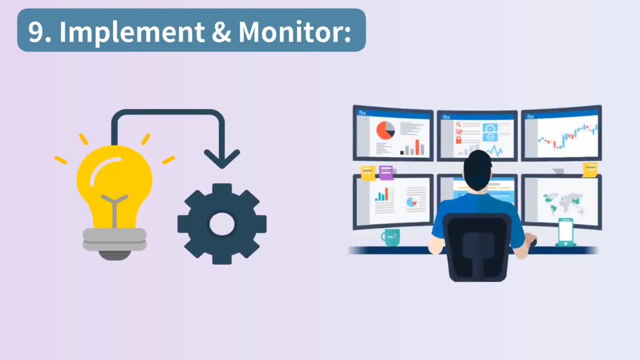 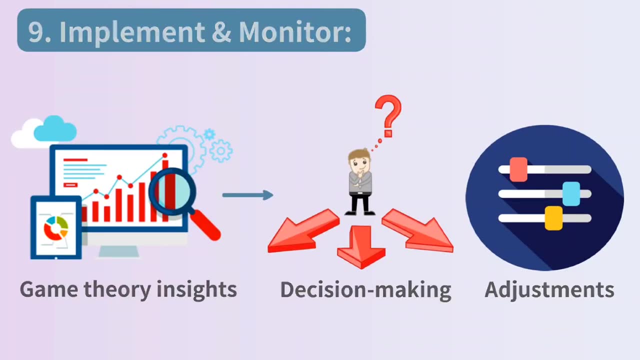 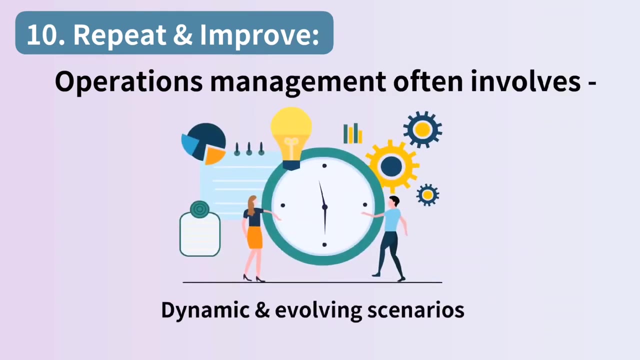 competition negotiation or a mix of these approaches. 9. Implement and monitor. Put the chosen strategy into action and closely monitor the results. Game theory insights can guide ongoing decision-making and adjustments as necessary. 10. Repeat and improve Operations. management often involves dynamic and evolving scenarios. 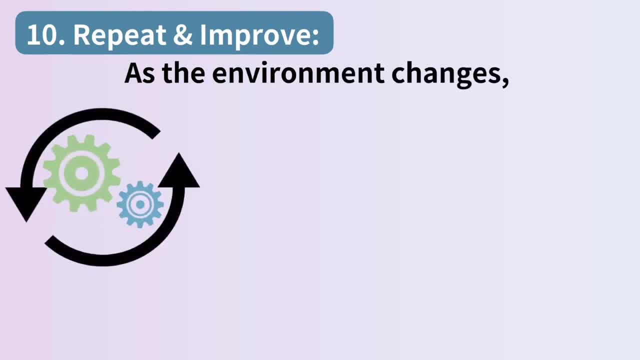 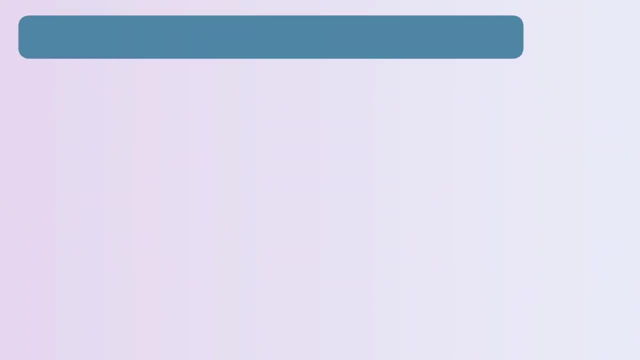 As the environment changes, you may need to repeat through the game theory process, updating strategies and analyzing new interactions. 11. Communication and collaboration. Effective communication and collaboration among the stakeholders are crucial. Game theory can help in designing negotiation processes and mechanisms. 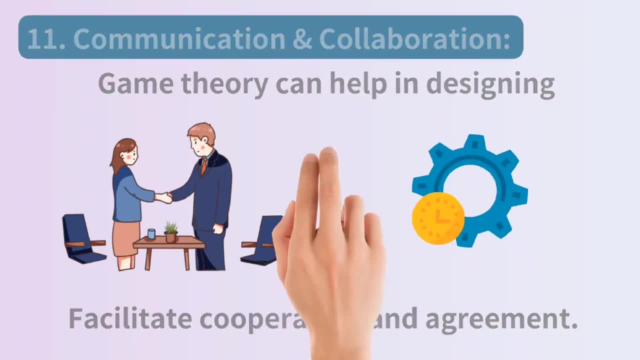 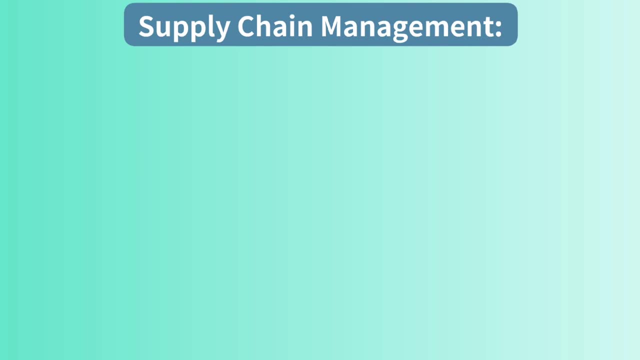 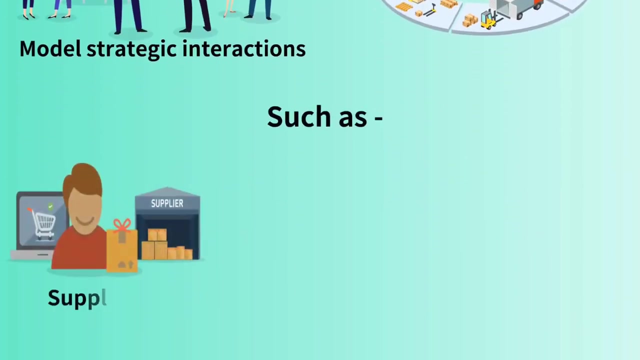 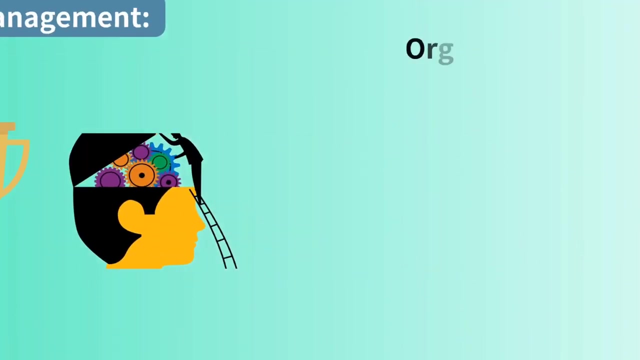 that facilitate cooperation and agreement. Applications of game theory in operations, research, Supply chain management. Game theory is employed to manage and manage the operations of, and model strategic interactions among, different entities in a supply chain, such as suppliers, manufacturers and retailers, By understanding the incentives and behaviors of each player. 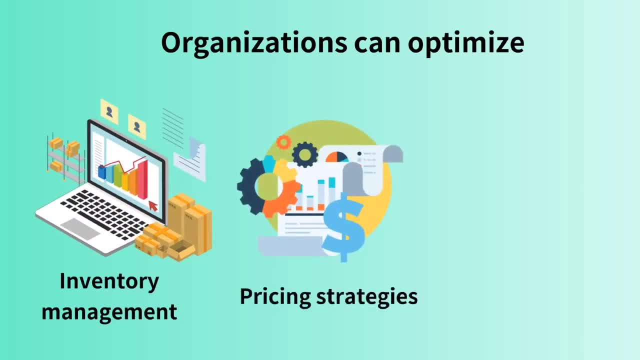 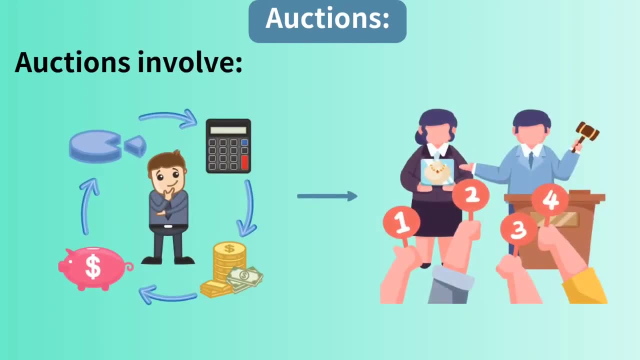 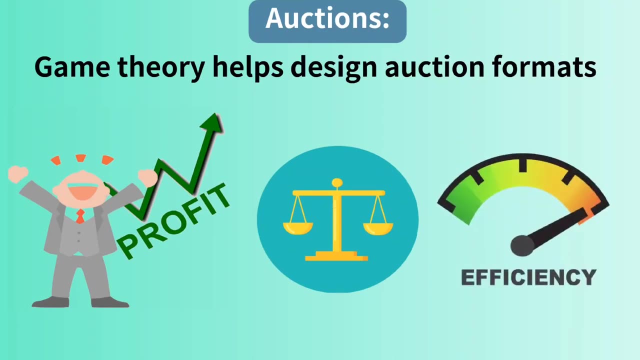 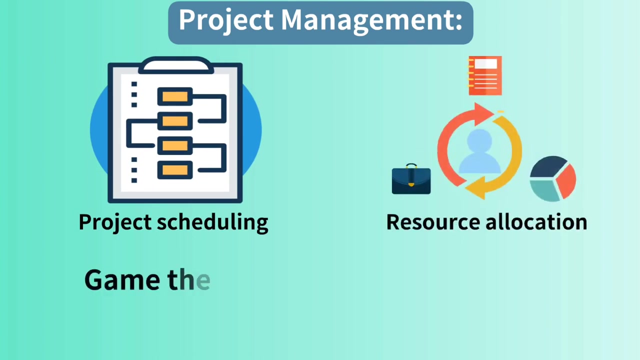 organizations can optimize inventory management, pricing strategies and distribution networks. 12. Auctions: Auctions involve strategic decision-making by bidders. Game theory helps design auction formats that maximize revenue for the seller while ensuring fairness and efficiency Project management. In project scheduling and resource allocation, game theory can be used to. 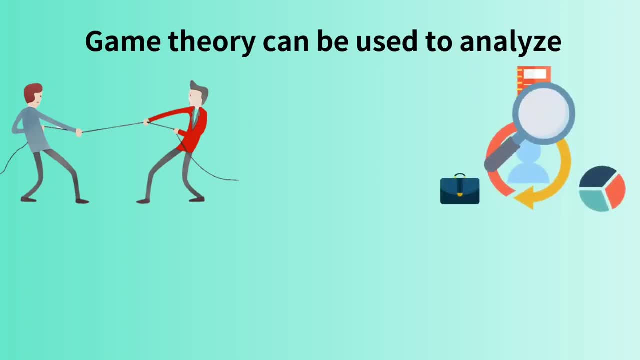 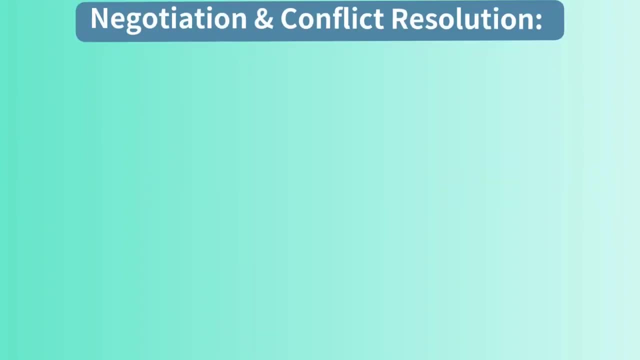 analyze conflicts of interest among project teams, helping to optimize resource allocation and task scheduling. Negotiation and conflict resolution: Game theory can be applied to model negotiations between parties with conflicting interests. This aids in achieving mutually beneficial outcomes in scenarios like labor disputes or international diplomacy.